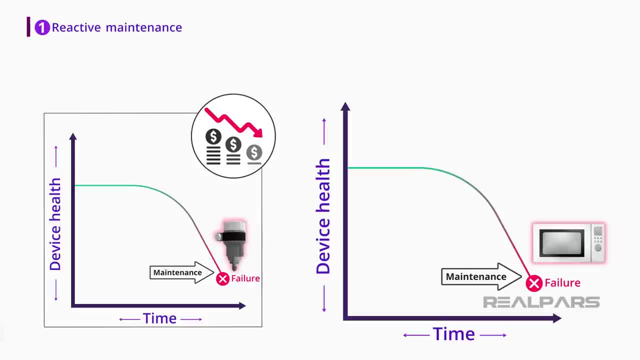 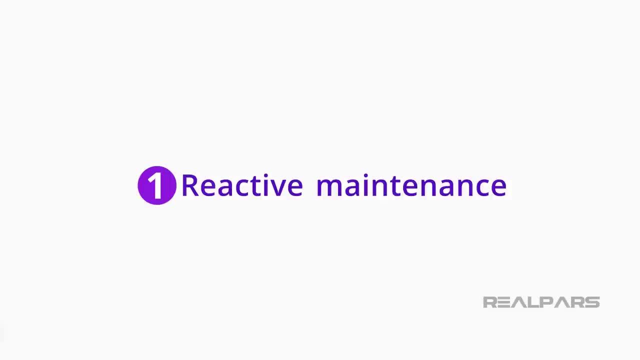 Or reactive maintenance may work fine for your microwave oven, but it is probably not the best choice for industrial processes. So what is the solution? The solution is to use preventive maintenance. With preventive maintenance, you try to perform maintenance for the device long before the device gets to the point of failure. 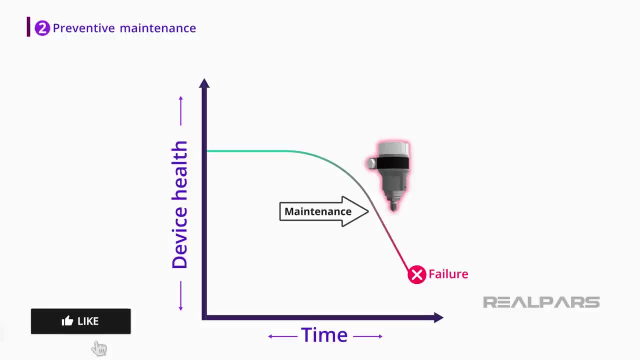 For example, you can check the pressure transmitter regularly and before it gets to the point of failure, to make sure that there won't be any sudden interruption to the industrial process. However, this is not very cost-effective. Why, you ask? Because by performing the maintenance early, you waste device life that is still usable. 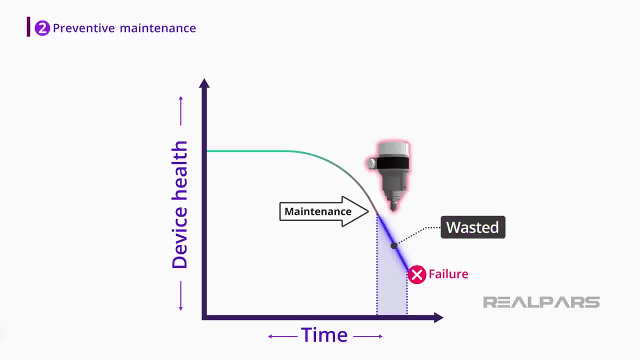 This is the time that we could still use the device without any maintenance, but now we're losing that because of early preventing maintenance. This is where predictive maintenance can help, As the name suggests, with predictive maintenance, you predict when the device fails. 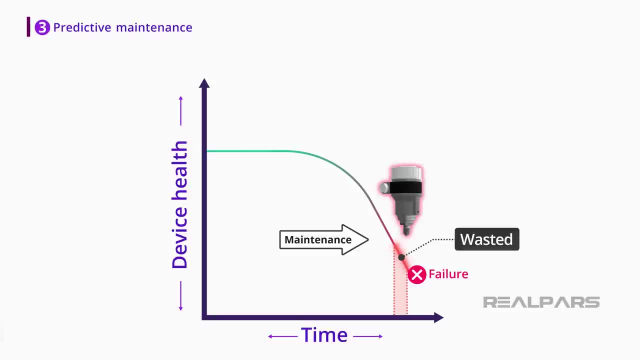 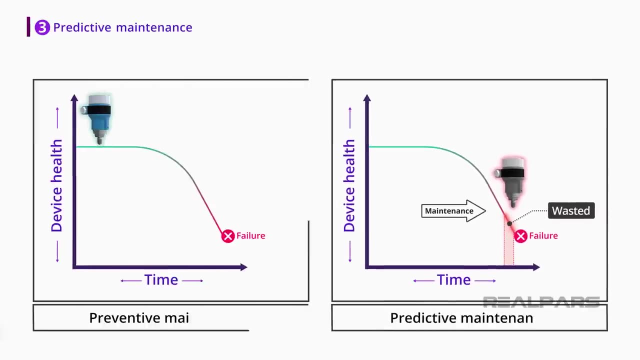 and schedule maintenance during that time. You can do this just before that. Following this process, you minimize the device or machine down-time and maximize its lifetime. So with preventive maintenance you solve the down-time issue and prevent it from happening, but you lose on device lifetime, meaning the time you could use the device without any issue. 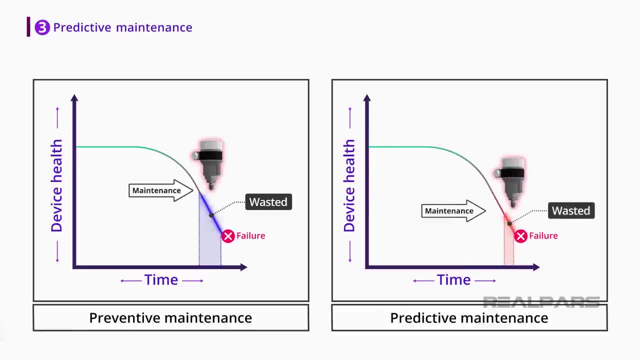 However, with predictive maintenance, not only can you solve the device down-time issue, but there will also be little to no wasted device life lifetime. This is cool, right? It's like you're cheating. You know when the device might fail, you wait and play it cool and then, right before the device fails, you perform. 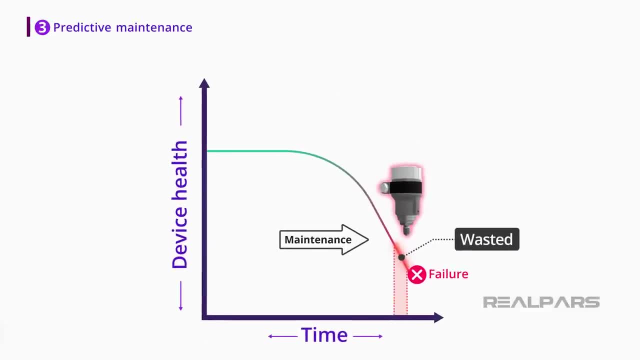 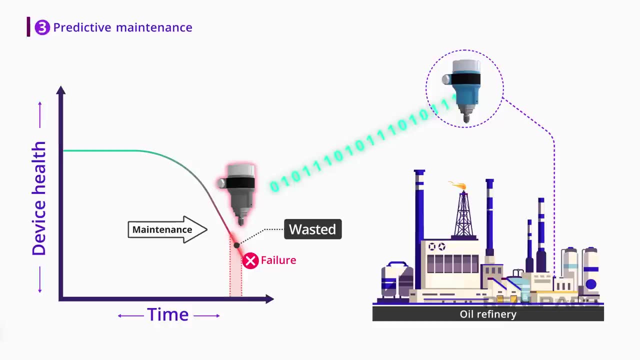 maintenance on it. Now you may ask: how are we doing this? How can we predict when a device fails? Well, this is simply done using the previous data that we have collected from a similar device in the past, For instance, with the pressure. 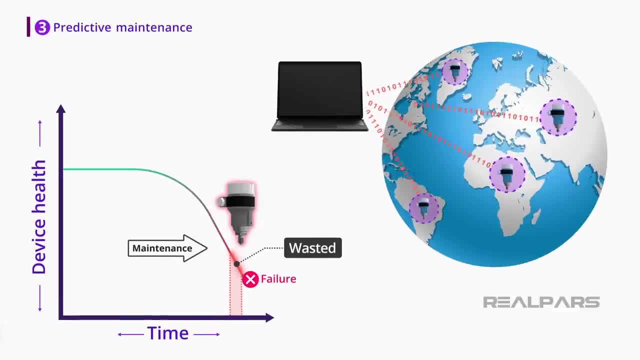 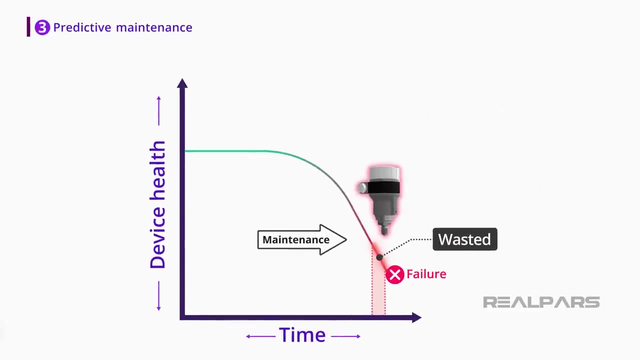 transmitter example. there are already thousands, if not millions, of similar devices installed all over the world from the same brand. By analyzing the available data from these current devices, we can pretty accurately predict when a similar device fails. The fancy term that we currently use- or maybe overuse- for utilizing this data is AI or 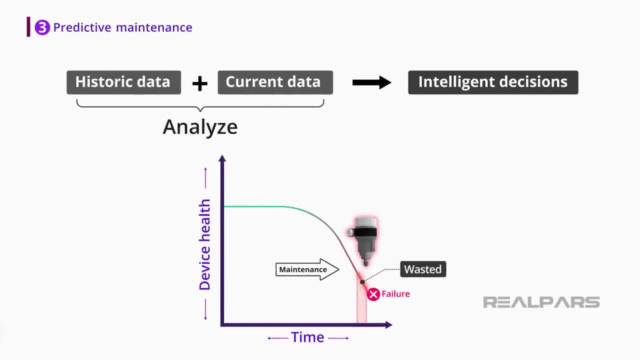 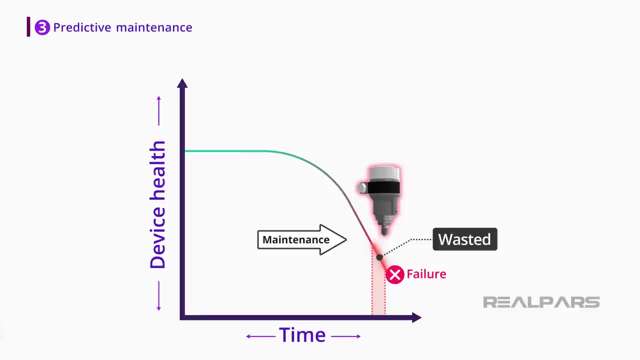 Artificial Intelligence, But the basic principle comes down to analyzing his story. One of these intelligent or smart decisions that we can make is to predict when a similar new device will fail in the future and perform maintenance right before that. Hence, predictive maintenance. 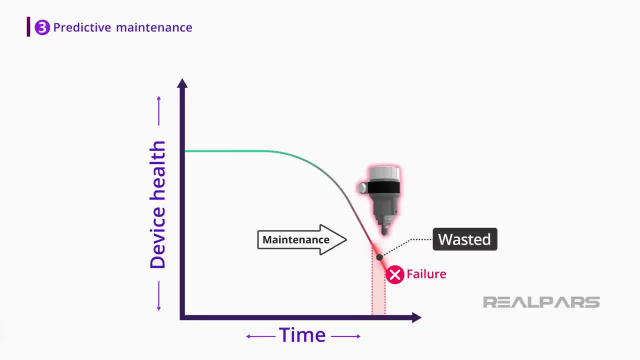 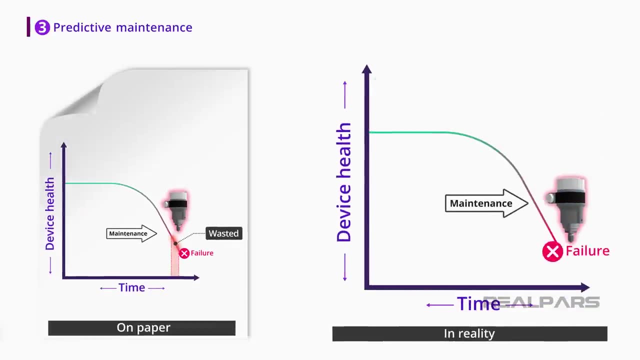 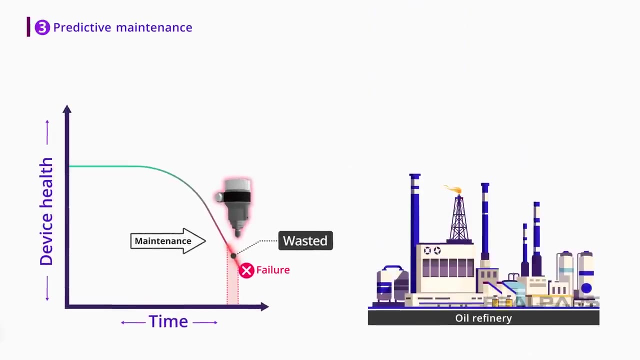 Now, at the time of posting this video, we're still at the beginning phases of this whole predictive maintenance stuff. You may argue that this will never work as accurately as it sounds on paper. Word is very expensive to implement, and you may be right, my friend. 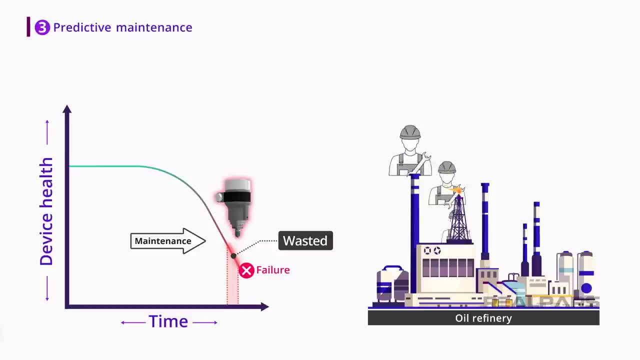 With all the recent years' advancements, we- I mean people in industry- are still in the learning and adaptation phase of predictive maintenance. So it may take a few years, or maybe a couple of decades, for us to properly transition from preventive maintenance to predictive maintenance. But hey, we're getting there. 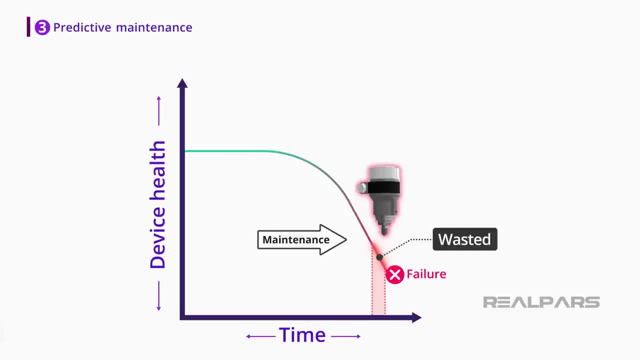 It may be off the topic here, but as I'm working on this video, I'm going to be talking about the concept of predictive maintenance throughout the entire timeline. Here I have some interesting thoughts that I'd like to share with you. What if we could? 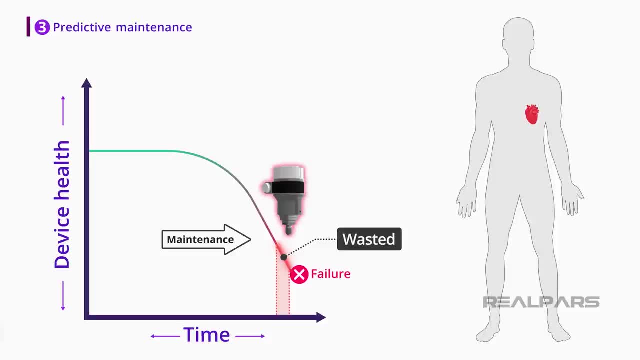 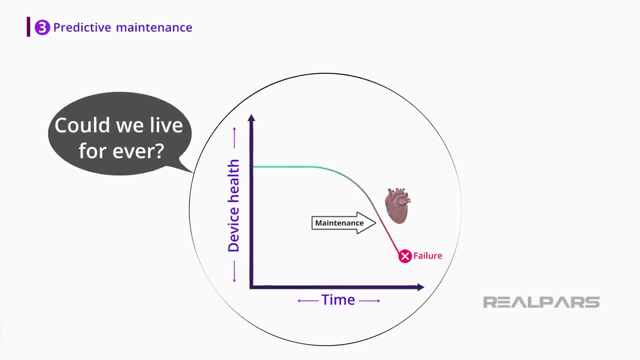 apply this whole concept of predictive maintenance to human body organs. I mean, what if we could replace a heart before it fails, for example? Could we then live forever? What if aging is a disease? Consider how the world would change if we could live forever. 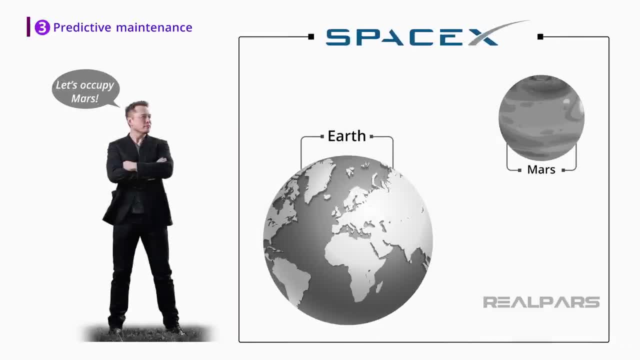 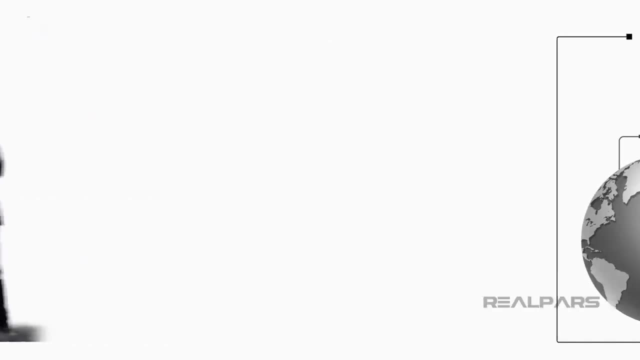 The plan that Elon Musk and SpaceX have started for making humans multiplanetary seems in line with living a considerably longer life. Let me know in the comments below what you think of this. Okay, enough of crazy futuristic ideas, Let's get back to the present time. 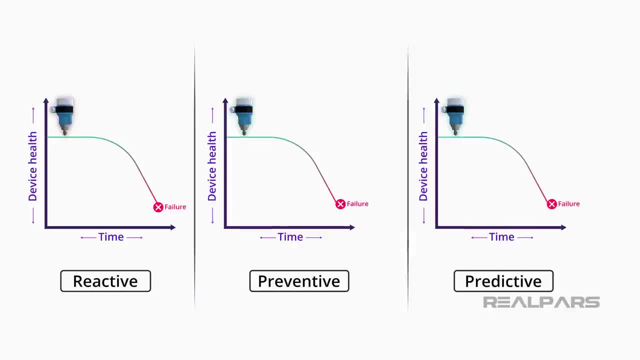 In summary, we have three types of maintenance: Reactive, preventive and predictive. Reactive maintenance is when you wait until the device fails and then you fix it. This causes your production line to stop and results in financial losses. To prevent this, you can use preventive maintenance. This is when you 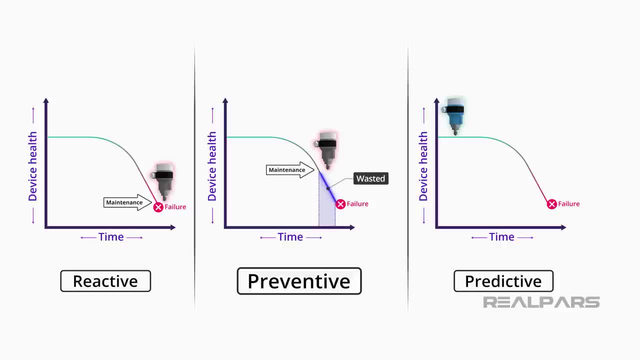 perform regular checks and maintenance before the device fails. But the challenge with preventive maintenance is by performing the maintenance early, you waste device life that is still usable. With predictive maintenance, however, you can predict when the device fails and schedule maintenance right before that.